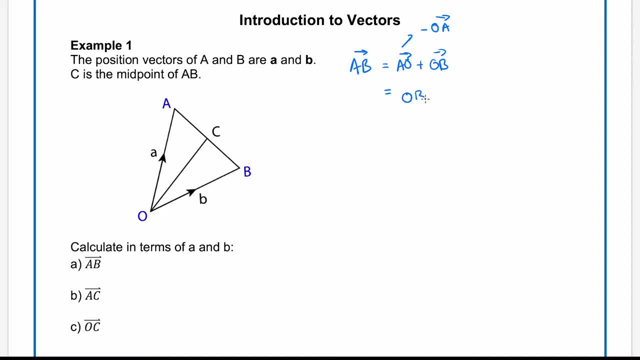 So now we can tally this up as O to B minus O to A, And we've been told that O to B is B and O to A is A. So we can write A to B as B minus A. So now the vector A to C. 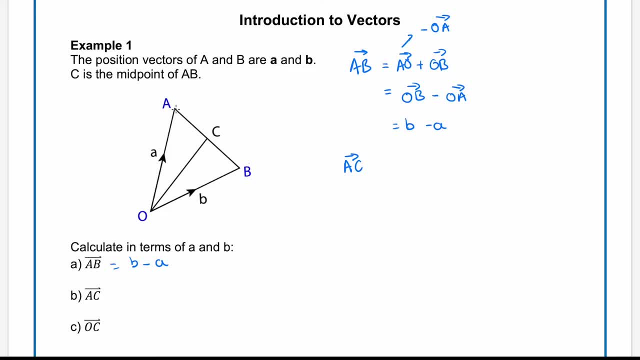 we've been told that C is the midpoint of A to B. so A to C will have half the magnitude but the same direction as A to B. So we can write it as one half of the vector A to B. And we've already worked out A to B as B minus A, So one half. 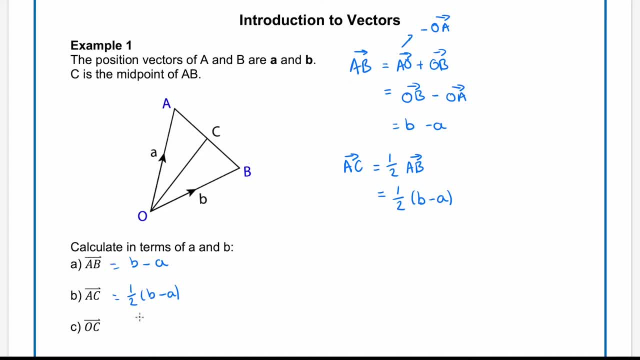 of B minus A. For question C, the vector O to C, where we can go to O to C by going from O to A to what's in the middle of terms, same as O to A, if we want to apply it, And A to C. we've been taught. 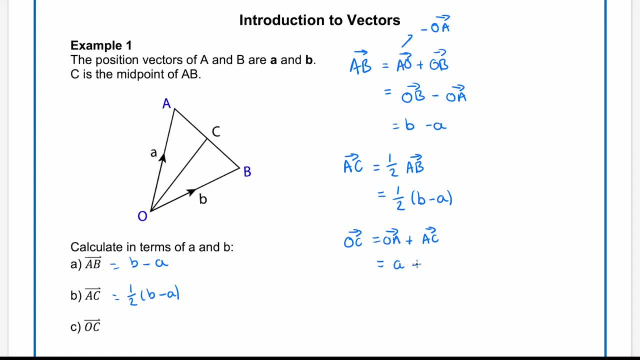 that we can: a followed by A to C, followed by A to C. O to A, we've been told is A and A to C. we've worked out they're kind of The first time. the answer is: A значит an Fn half of a. We're using collectively a terms, so one half of a plus one half of b and we can factorize. 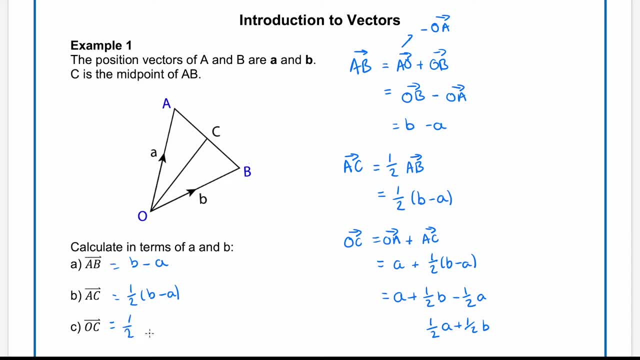 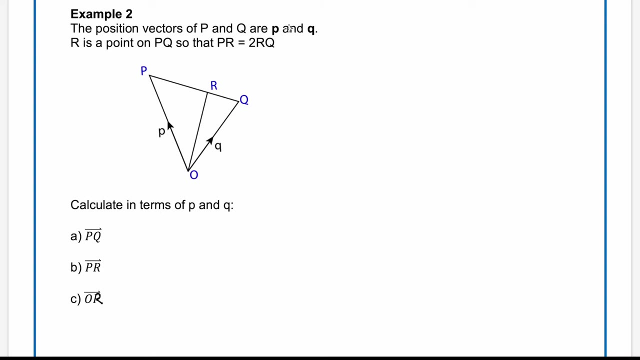 up the half to make it a bit tidier. so one half lots of a plus b. Okay, let's try the next question. So for question two, we've been told the position vectors of p and q are p and q when these vectors are given in bold and r is a point on p to q, so that p to r is double the. 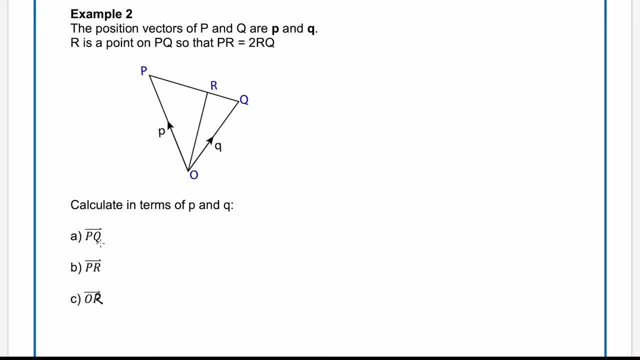 length of r to q and we've been asked to work out p to q in terms of these vectors. So p to q will be equal to p to o, followed by o to q, and we know that p to q is the length of r to q. 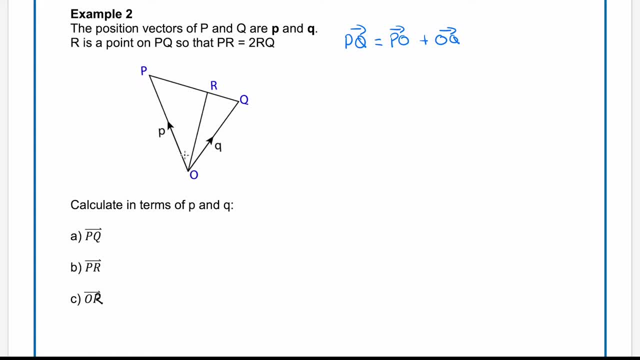 and we know that p to q is the length of r to q and we know that p to q is the length of r to q. So p to o is the same magnitude, but the opposite direction of o to p, so we can write this as o to q. 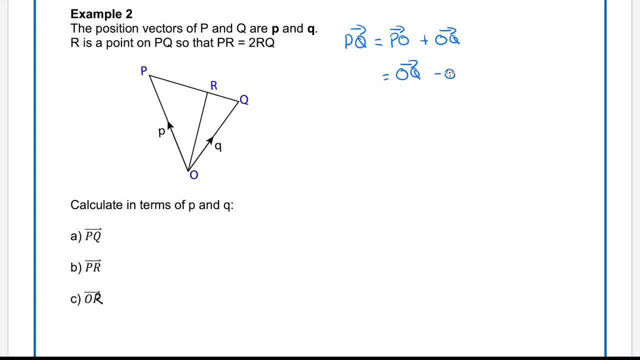 minus o to p. We know o to q is q and o to p is p, q minus p. and for question b, the vector p to r. well, we've been told that r is a point of p q, so that p to r is double r to q. so we can write this as: 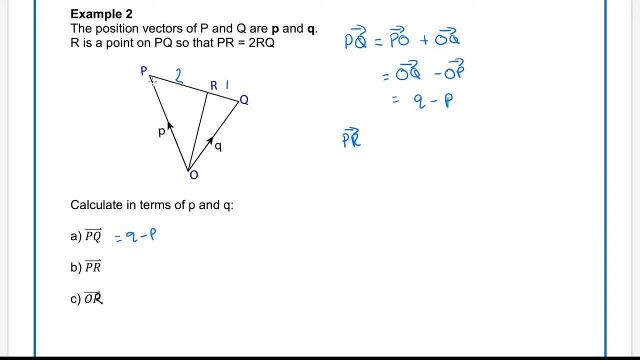 two parts and this would be one part. so we've broken up the line p to q into three parts, and p to r is two of them. so that would be two thirds of r to q, which is two thirds of q minus r to q and the question c, o to r. well, we can go from o to p, followed by p to r. 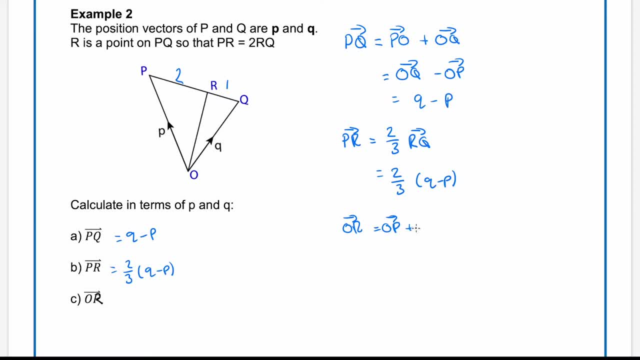 so o to p plus p to r. so o to p, we know, is p and p to r is two thirds of q minus p, so let's band out these brackets. so p to p is two thirds of q minus p, and p to r is two thirds of q minus p. 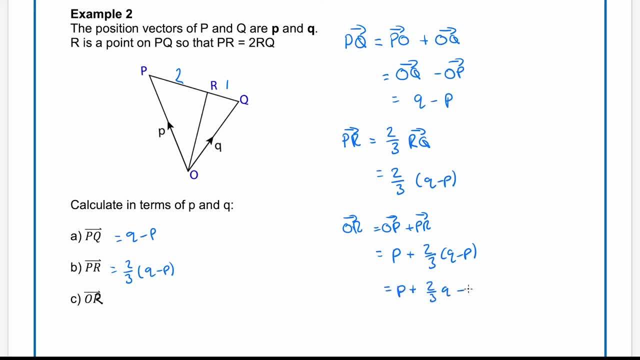 plus two-thirds of Q, minus two-thirds of P. We can collect the P terms, so one-third of P plus two-thirds of Q, And we can factor that with third, so one-third lots of P plus two-Q. Okay, let's try another question. Okay, so for example, three. we've been given this. 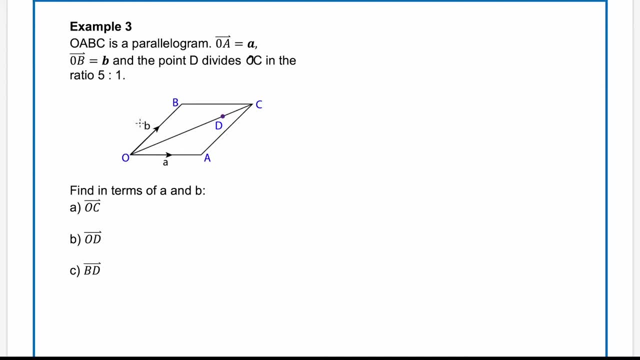 parallelogram. we've been told that O to B is a vector of B, O to A is a vector of A and that the point D breaks up O to C in the ratio five to one. So we're going to work out the vector O to C. 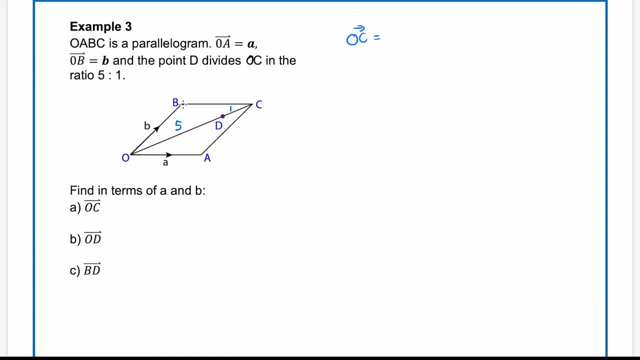 And this is O to B plus B to C. But because it's a parallelogram, we know B to C has the same direction and the same magnitude as O to A. So we can write B to C as a vector of A. So O to C, O to B plus B to C. O to B, we know, is B. 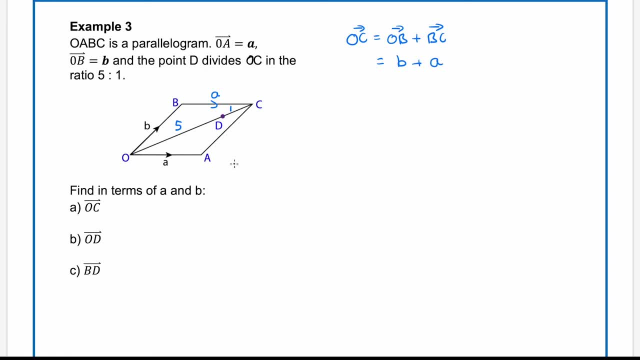 And B to C is A, So we have A plus B. So for question B, the vector O to D. well, because we've broken up the line O to C into six parts, we know O to D is five of them, So this will. 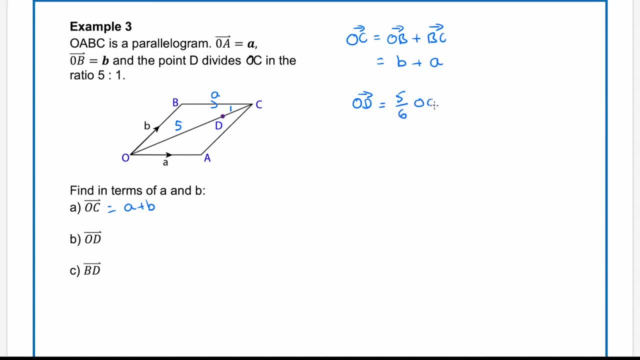 be five-sixths of the vector O to C, Which is five-sixths of a vector. So we need to, which is 5, 6 of b plus a, and now vector b to d, which is this vector. here we can go from b to o. 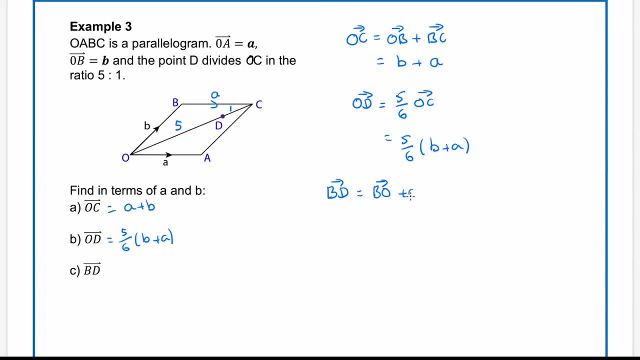 plus o to d, b to o. i'm going to write as minus o to b, so o to d, minus o to b. o to d. we've worked out as 5, 6, lots of b plus a and o to b. we know is b, so minus b. 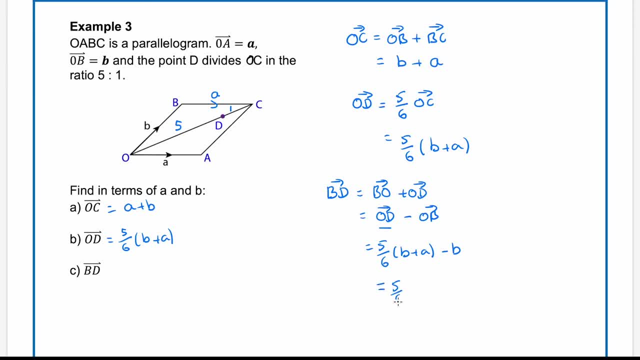 we can expand this bracket, so we have 5- 6 of b plus 5, 6 of a minus 6- 6 of b. so we have our a term: 5, 6 of a, and then 5, 6 minus 6. 6 is minus 1- 6 of b. 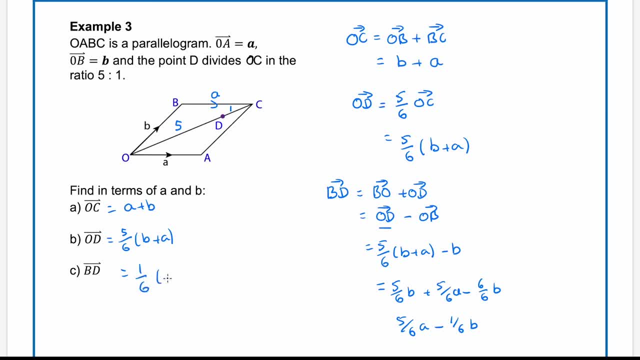 so we can factorize out the 1- 6 and we have 5 a minus b. okay, thank you for watching and i hope you found that useful. thanks again and take care.